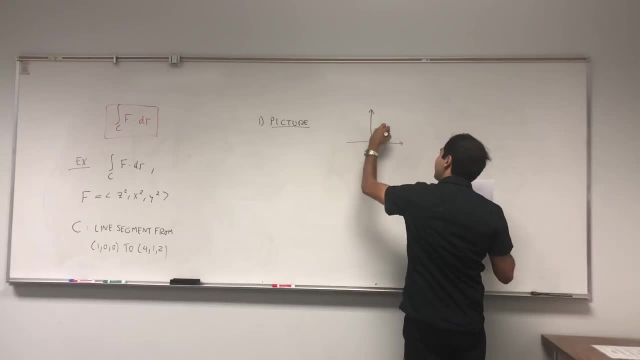 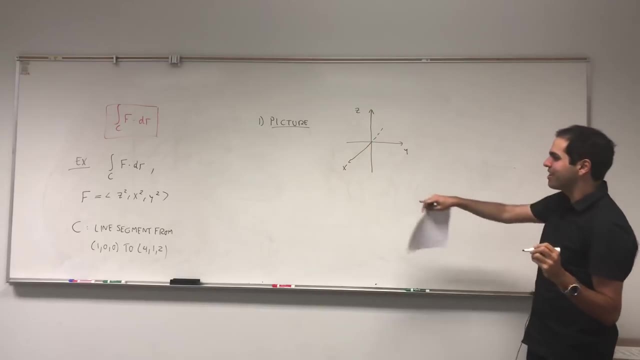 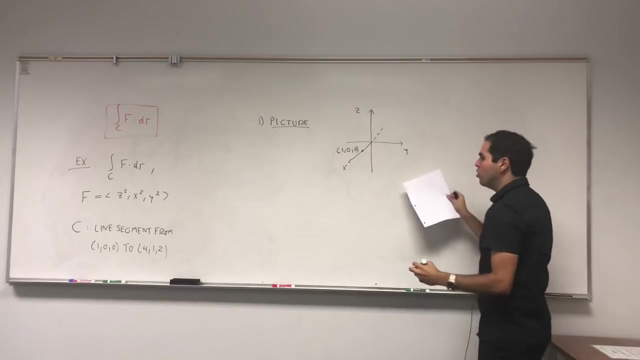 It's very, very important Because it seems like an algebraic course, but it's actually a very geometric course. I think that's what makes the class so hard. So we have the line segment from 1, 0, 0, so here, for example, to 4, 1, 2, which maybe looks like 4 1, 2, let's just put it here: whatever. 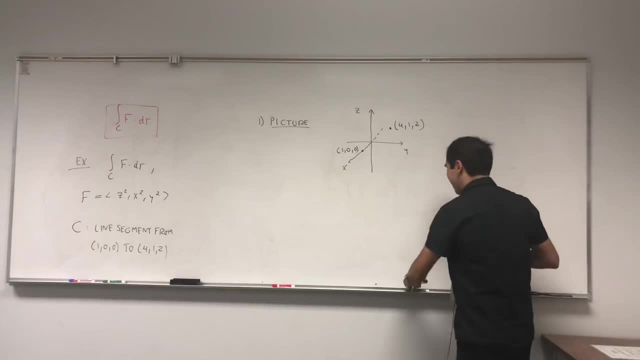 Just to give a rough idea of what's going on. And we have this line segment, segment C, here. It's just a line segment connecting the two points in this direction. and again, directions are important and essentially- and I'll talk more about that in a second- what you want to do, you want to sum up the values. 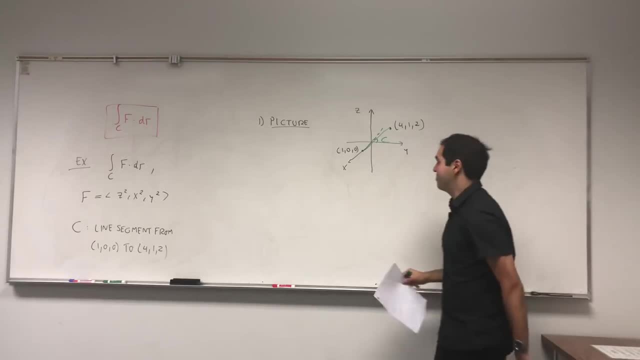 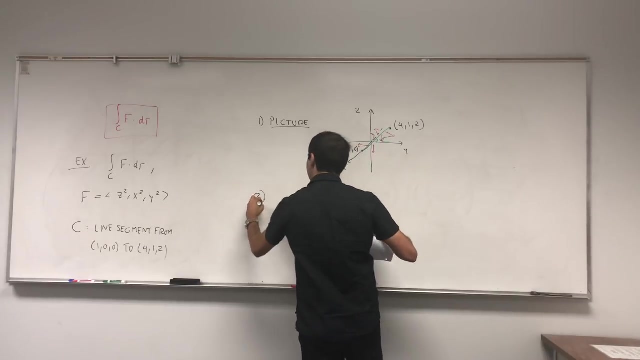 of those vector field over this segment C. so in other words, you have a bunch of arrows pointing everywhere. essentially wanna sum up all those arrows, which doesn't make sense, but it turns out there's a way of making it make sense. and again I want to emphasize: the most important thing in vector calculus is 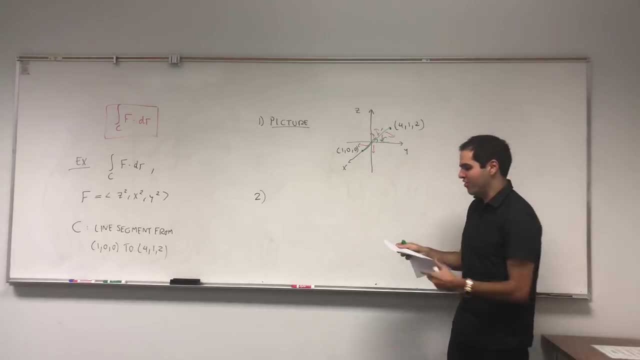 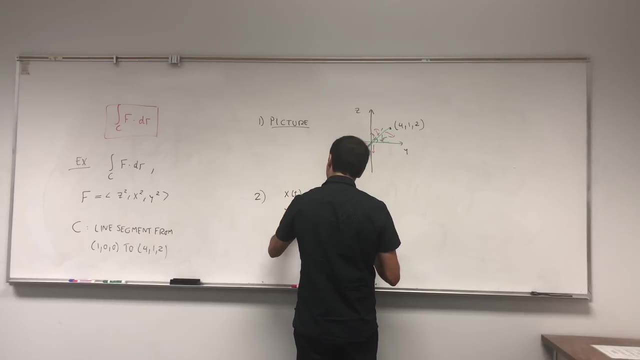 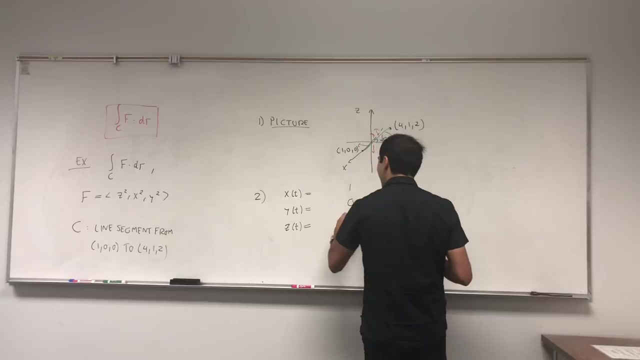 just parameterizing your curve or your surface. so now let's just parameterize our sample's for C, that line segment, So x of t, y of t, z of t. And here's a neat thing: There's actually a very systematic way of parametrizing line segments. So you put your points here: 1,. 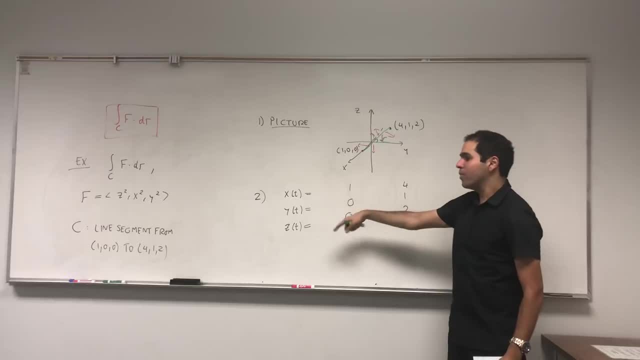 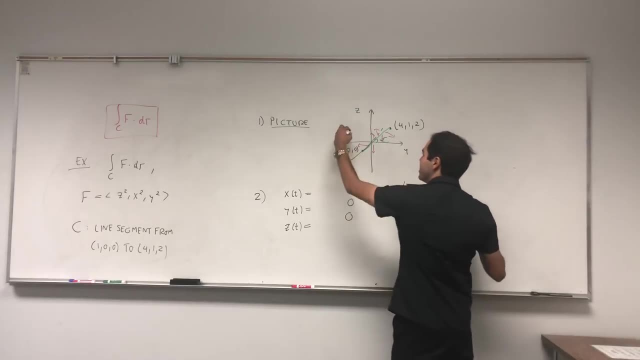 0, 0, 4, 1, 2, and then you put what I call an on and off switch. So at the beginning, at t equals to 0, you want to have the point 1, 0, 0. That's why you put 1 minus t's here. 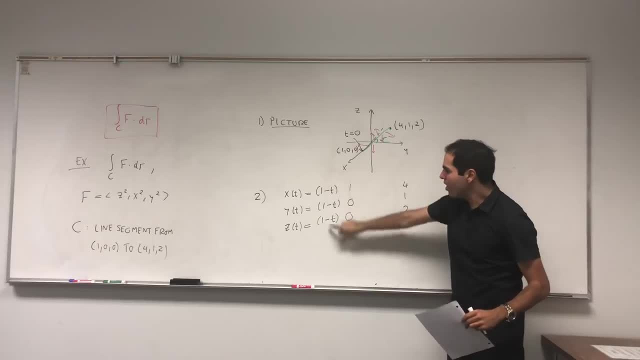 Because, again, at t equals to 0, we want this to be 1, because we want to start at 1, 0, 0. Whereas at t equals to 0, we don't want to have 4, 1,, 2, so you put t's here. 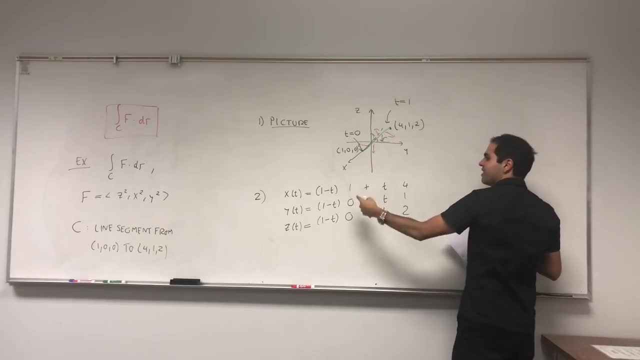 And essentially that's why I call it an on and off switch, because here you put it on and you get 1, 0, 0. And here you have it off, so 0, 0, 0. But at t equals to 1, it's the opposite. You start. 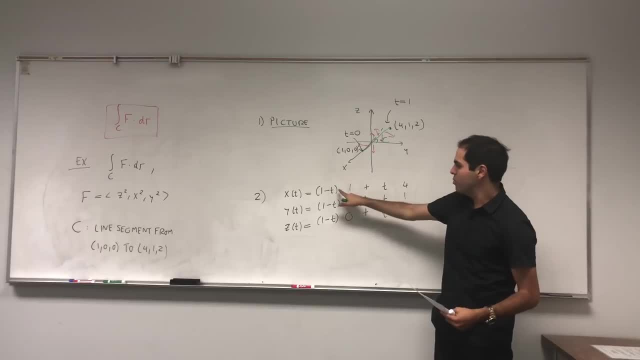 with 1.. You don't want to have 1, 0, 0.. So you put 0, 0, 0 here. But here you do want to have 4, 1, 1, 2, so you put 1, 1, 1.. 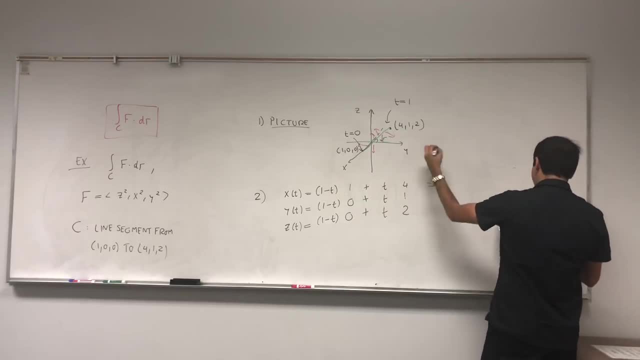 You can simplify this: That's 1 minus t plus 4t, so 1 plus 3t. Here we have 1t, and here we have 2t, And we get it from 0 to 1, as I said. 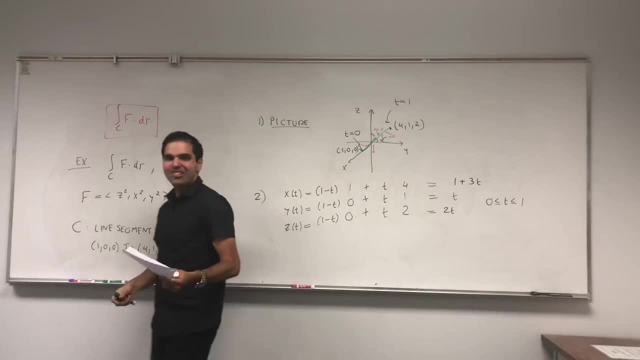 You want to start here and end here. By the way, 2t it's such a cute word. It means parrot in Farsi, so that's why it's like a 2t, except here we have 2t. 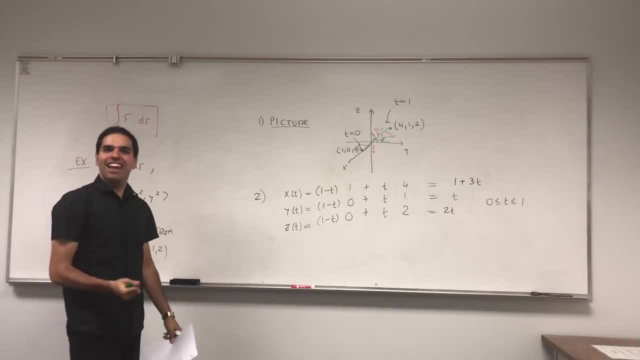 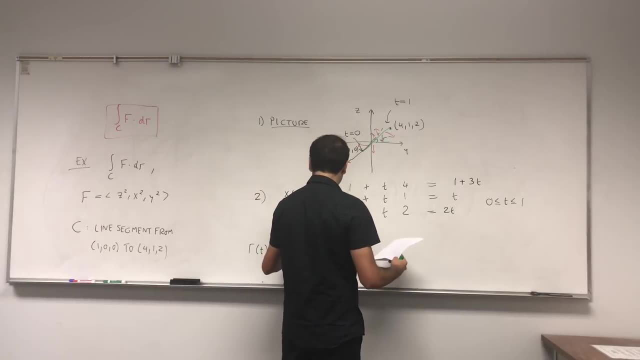 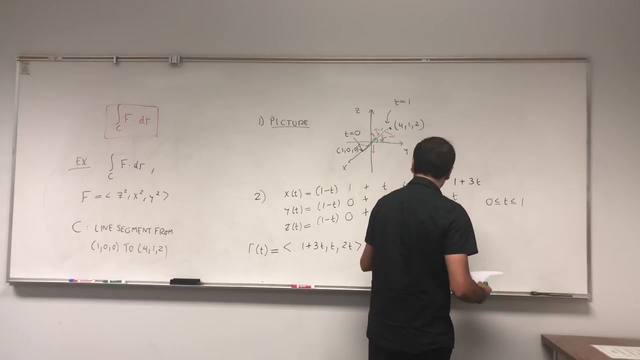 OK, and so here we have. points Turns out in vector calculus it's better to deal with vectors. So let's just combine that r of t is 1 plus 3t, t, 2t, And that's from t, from 0 to 1.. 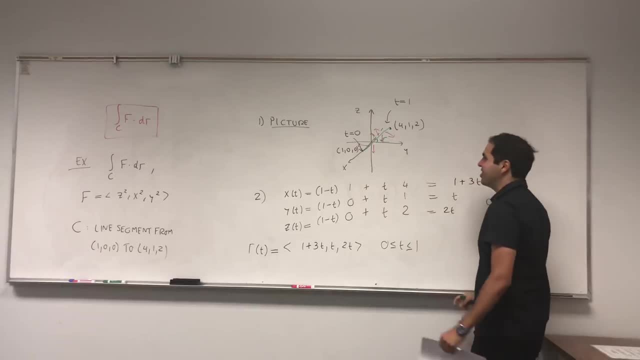 And r, not gamma. If I wrote it in cursive no one would read it. That's why I write it that way. And the point is: r of t is just a random point in vector. It's just a random point on this line segment. 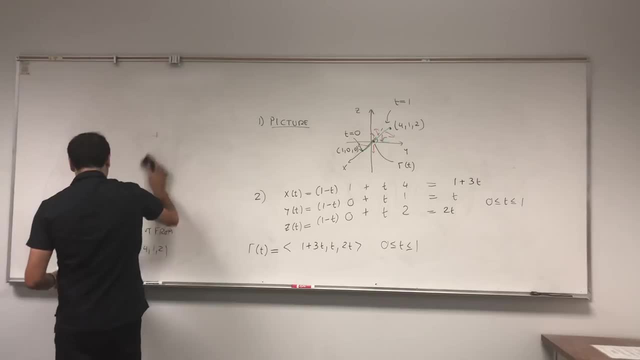 OK, and the question is now: how do we calculate that line integral? And you'll see, it's so beautiful. It's just this one idea. this one brings us way forward. So it's all based on this one clever idea. 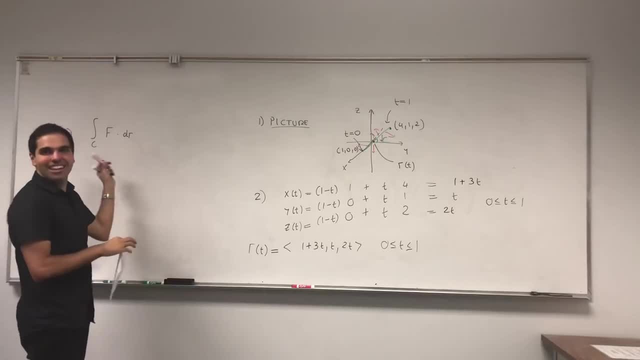 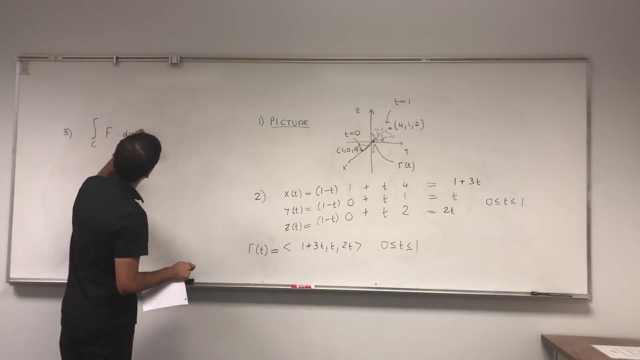 So f dotted with dr, and not Franklin D Roosevelt, That's someone else. Now here's the trick. Well, just as before we had dx dy, The trick was to multiply and divide by dt. Well, this works here too. 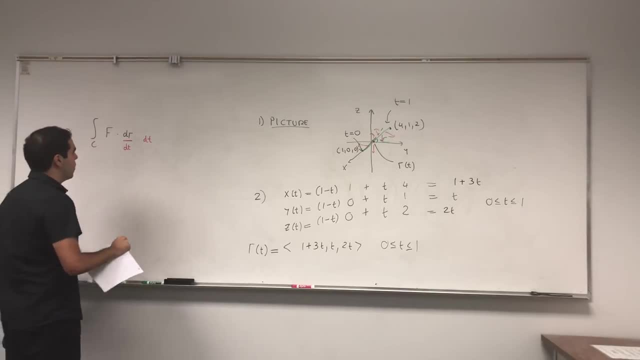 Take f dotted with dr. multiply top and bottom by dt, And what this becomes. Well, dr over, dt is r, prime of t, dt And f is just f. f at the point r of t And dot is dot. 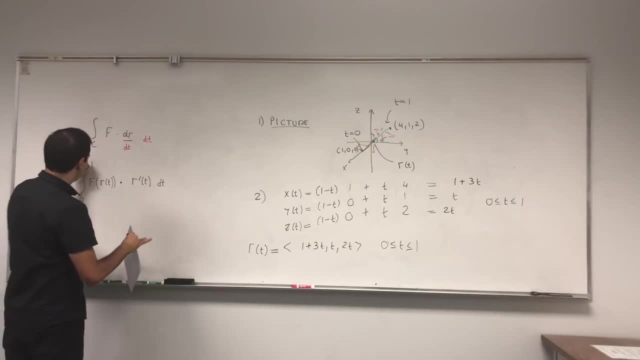 And because we're talking about t, you need t values from 0 to 1.. And that's again your formula. How cool is that? Now, what is f of r of t? It just means f, but with the values x of t, y of t, z of t. 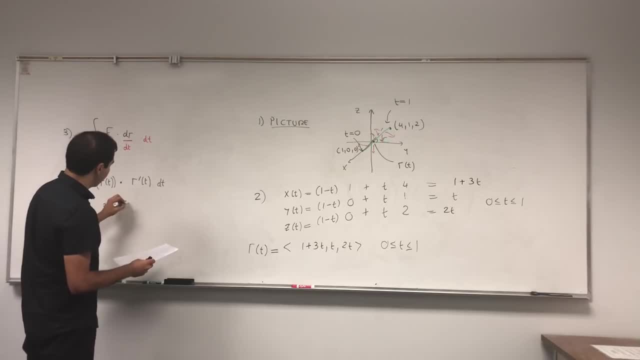 So remember, f was, I think, z squared, z squared, y squared, x squared. But here all you put is z of t squared, y of t squared, x of t squared, And you dot it with r prime, which is just x prime of t y. 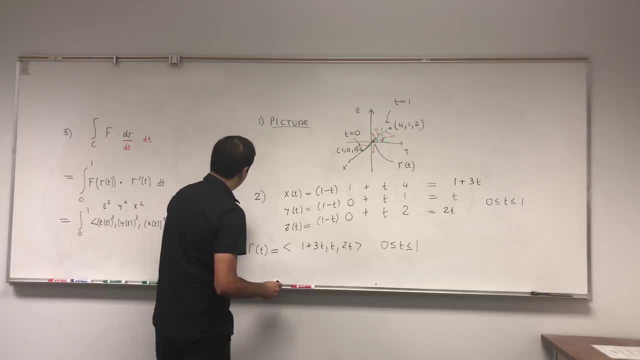 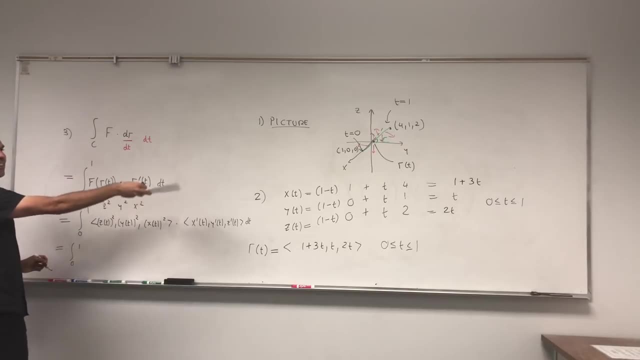 prime of t, z, prime of t, dt, And once you have that, you just use x, y and z. So z was 2t, so it's 4t squared. y was t, so t squared And x was 1 plus 3t squared. 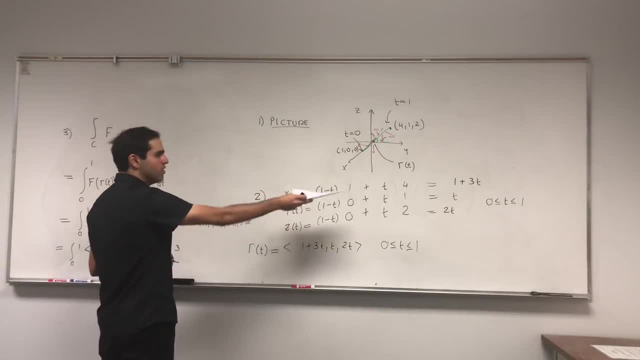 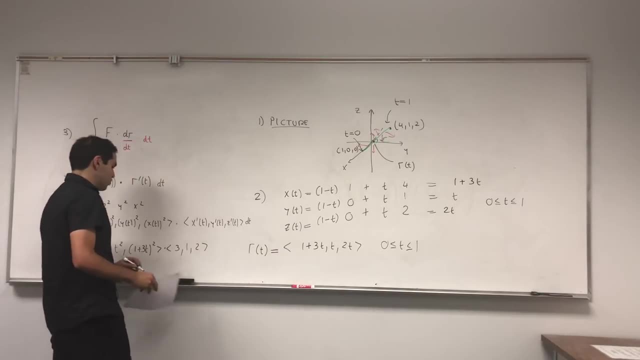 And you dot it with all the derivatives. So the derivative of 1 plus 3t is 3.. The derivative of t is 1.. The derivative of 2t is 2. dt And in general you can have different values. 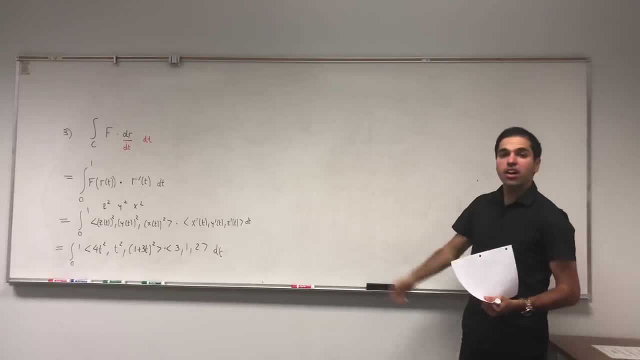 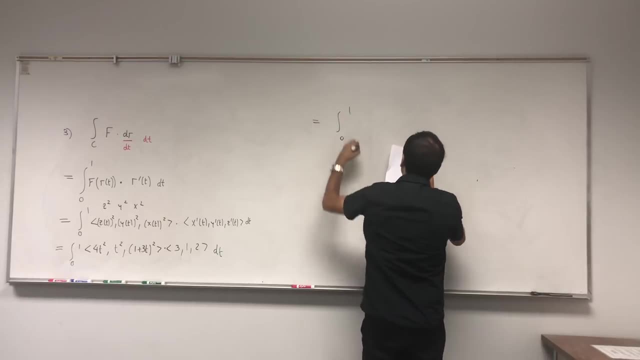 And the point is, yes, you have vectors, But because of the dot product, you just have a number And basically you just end up integrating a number. So it's integral from 0 to 1.. 4t squared times 3, which is 12t squared. 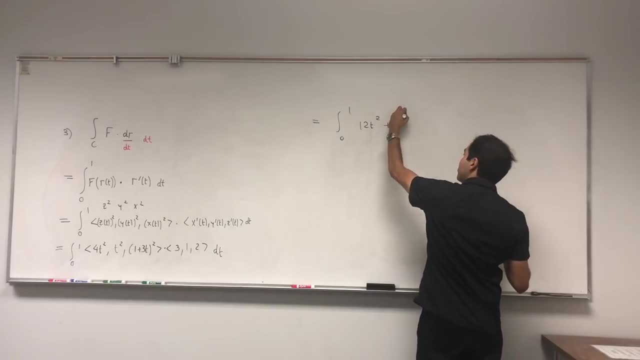 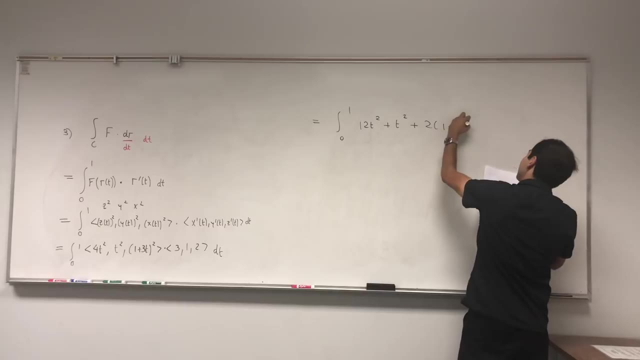 Plus t squared times 1, which is t squared Plus 2 times 1 plus 3t squared, That's 2 times 1 plus 3t squared dt. You calculate that So 12t squared plus t squared. 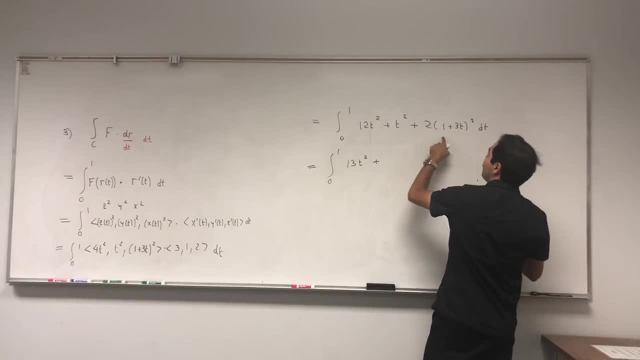 It's 13t squared. You fold that out, for example: So 2 plus 2 times 3.. That's 6 times 2.. It's 12t squared, That's 12t And then 3 squared. 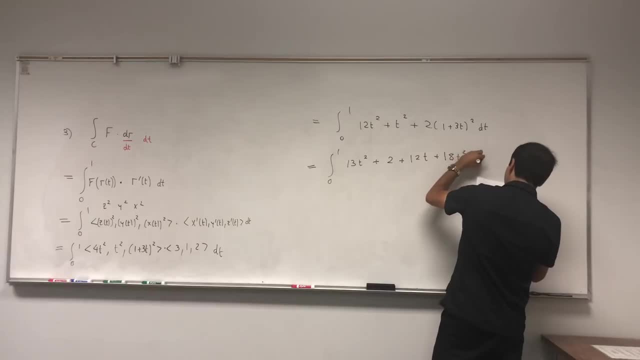 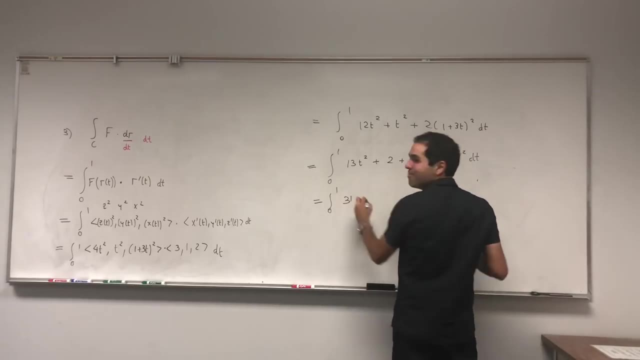 That's 9 times 2.. 18t squared dt And let's see 13 plus 18.. That's 31.. I'm not my age, Okay, 31.. Okay Plus 12t plus 2.. 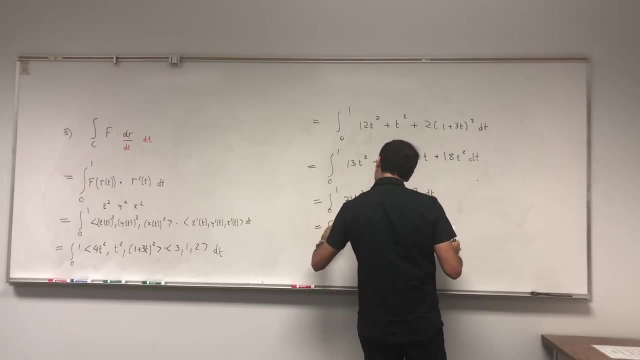 dt And you get 31q over 30q Plus 6t, squared plus 2t from 0 to 1, and that's 31 3rd plus 6 plus 2, and that's 8 plus 31 3rd and that's. 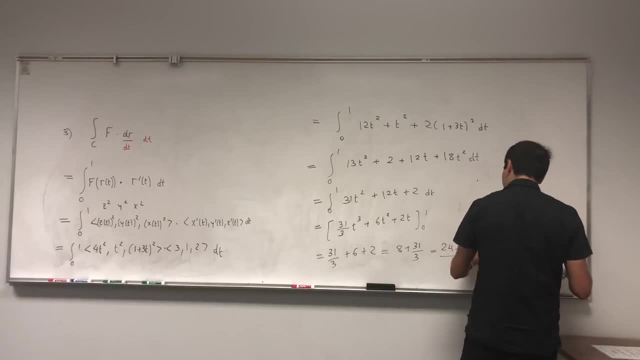 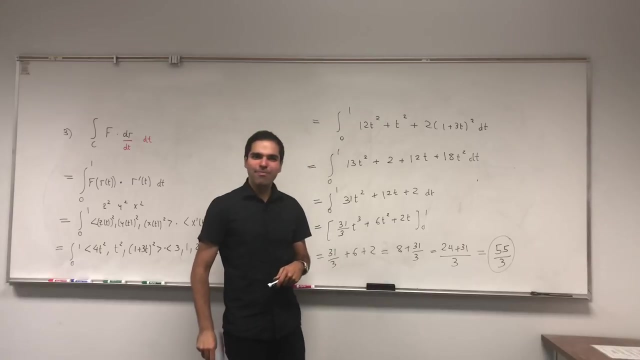 24 plus 31 over 3, and that's 50,. 55 over 3, and, by the way, 55, math 55, it's the very first class black pen and red pen took in Berkeley and that's actually how we met. 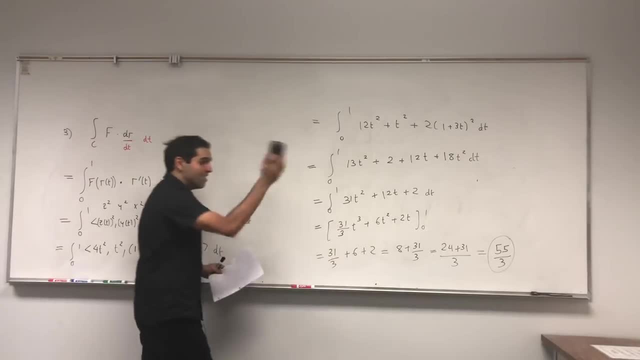 So how cool is that? So great? this line, integral f dotted with dr, is just 55 3rds. And, what's important to understand, you get a number because in the end you're integrating just a simple function. 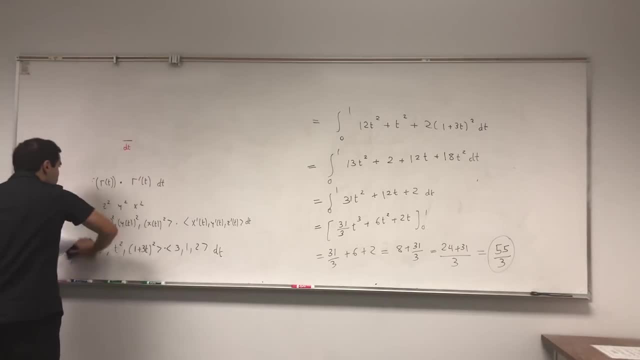 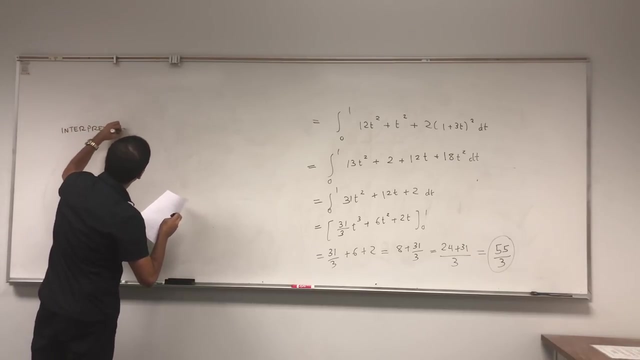 You're not integrating a vector. But it turns out you can still. You can still interpret it as integrating vectors. so let me give you a quick interpretation. And again, physicists they say: oh, it's just a work done by f over a curve. but again, 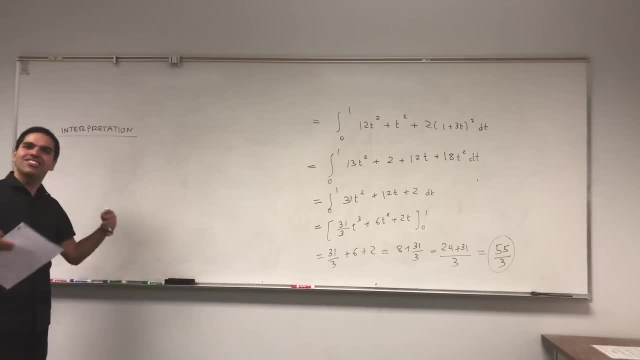 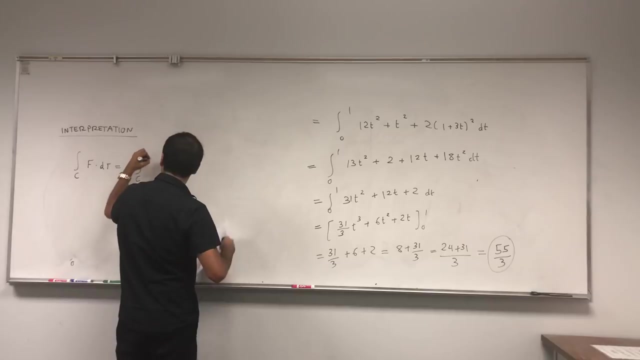 that doesn't mean anything to me, and I don't think you should just substitute the physics knowledge for math intuition, like some textbooks do. So what is f dotted with dr? And remember by what I said, it's just the integral of f of rt dotted with r, prime t, dt. 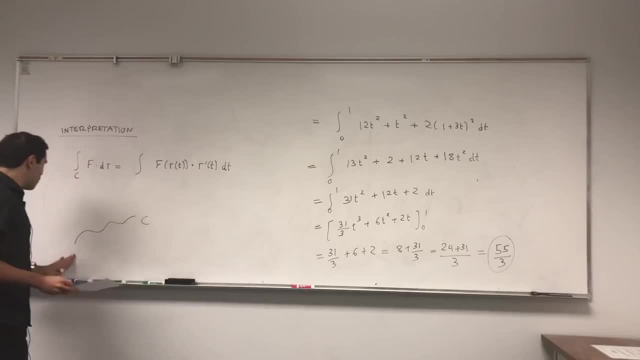 Now what is r prime t? So suppose you're at a point, remember r prime t, it's the tangent vector at that point, And so essentially what you're doing is at each point- Suppose this is f at the point rt. 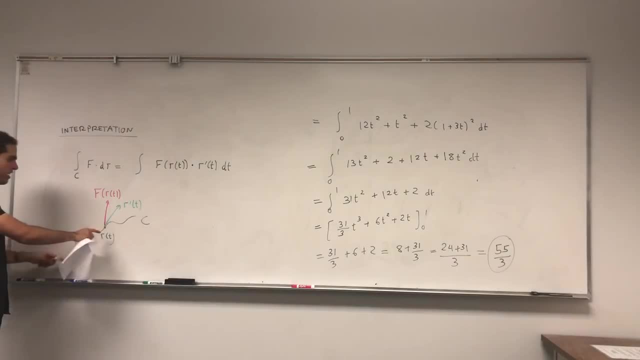 At each point you're summing up those little dot products, In other words, you're summing up small numbers. and what does each number tell you? Each number tells you whether f is in the same direction as the curve or not. 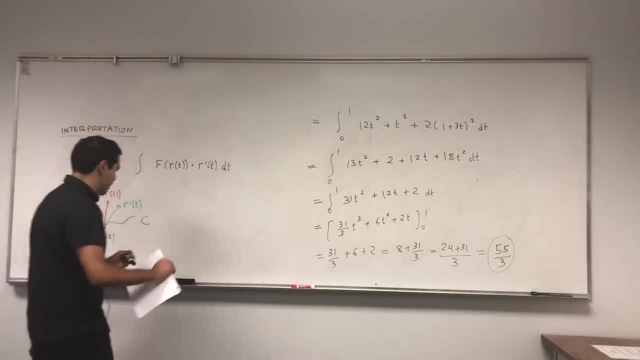 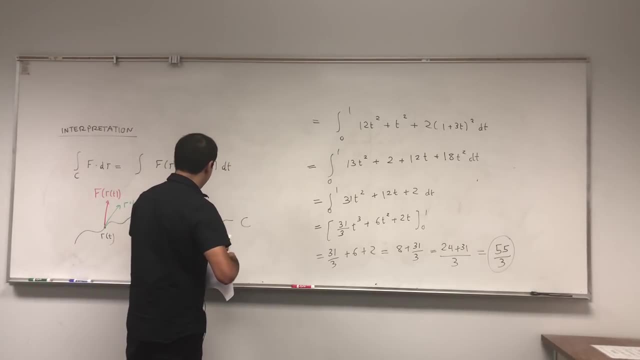 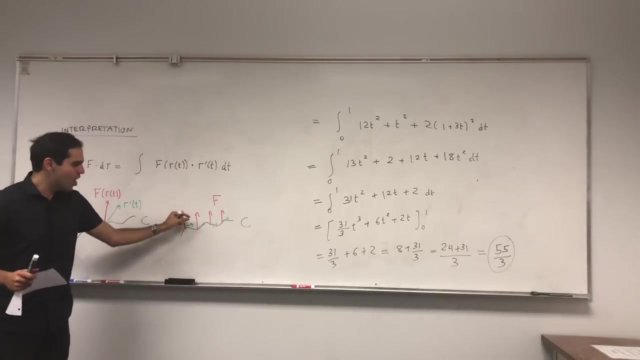 So, for instance, had a curve like this and at every point f is perpendicular to it, then f dotted with dr, well, it's pretty much 0. Because at every point you're summing up those little values, which is 0.. 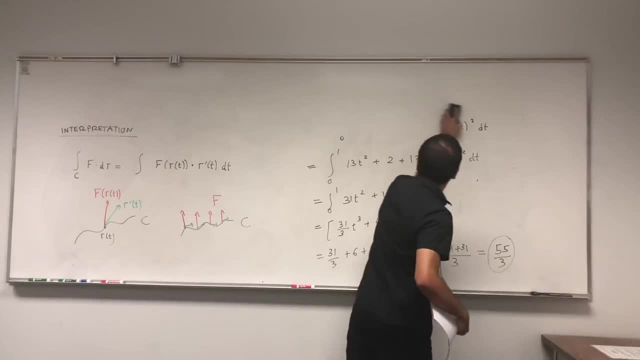 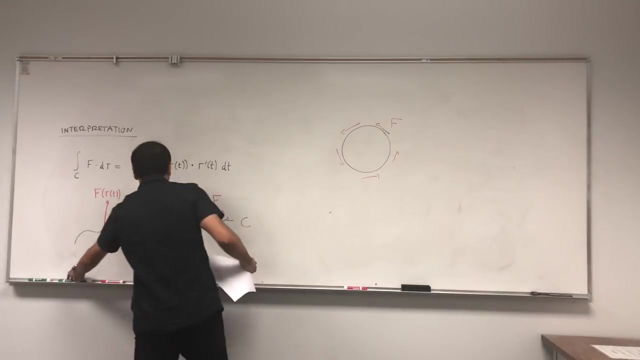 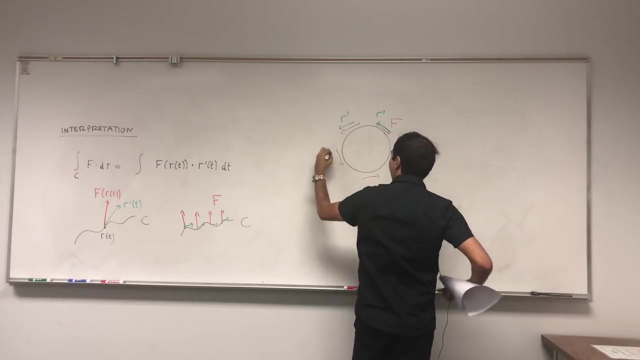 But suppose f sort of flows with the curve. So suppose, for example, you had a circle like this and f sort of moves along with the curve. And again let's draw the tangent vectors: r prime, r2.. r prime, r prime, r prime. 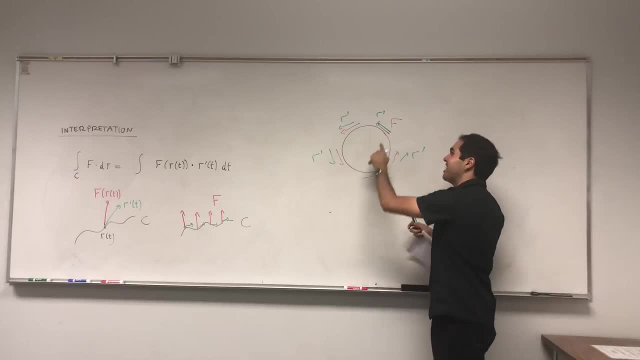 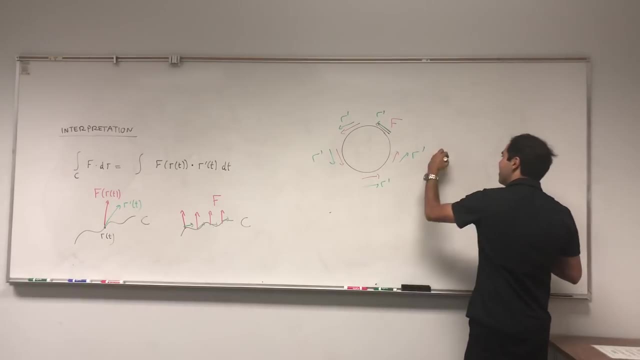 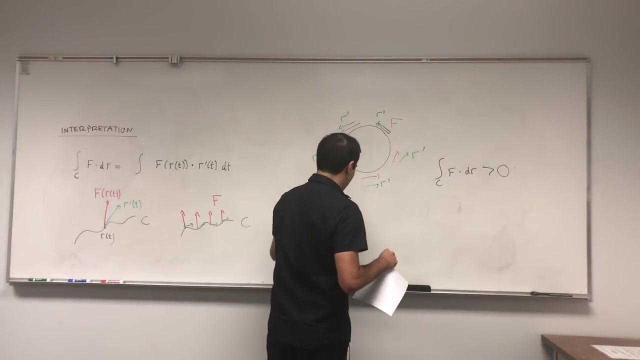 Then notice f dotted with dr is huge at every point because f faces the same direction as the curve And therefore in the end the integral f dotted with dr should be huge. so very positive. On the other hand, suppose the curve points like this: 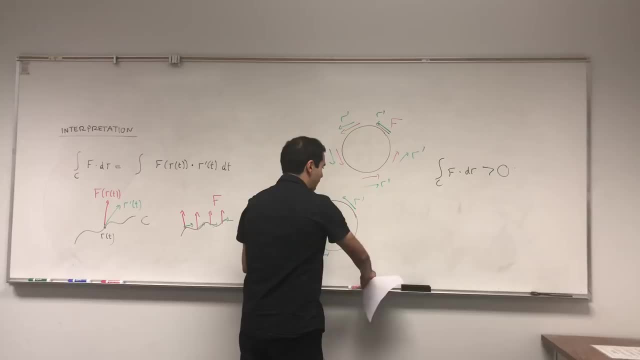 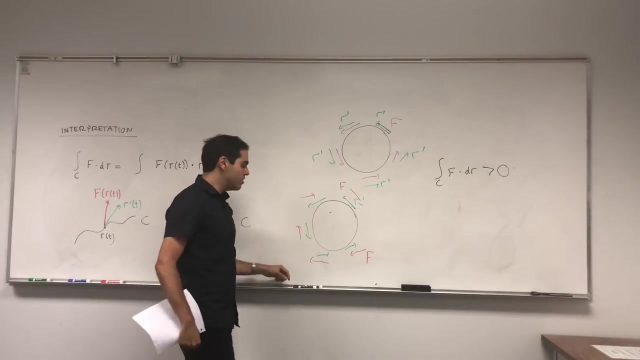 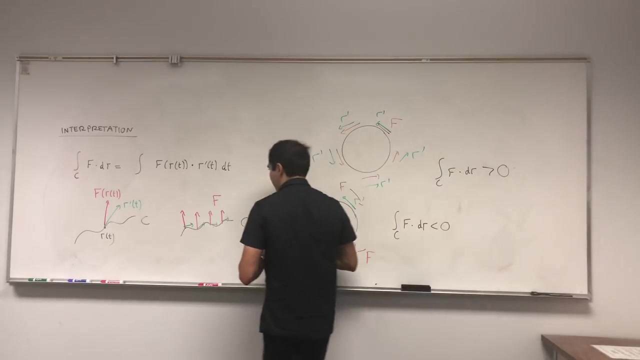 Suppose this is r prime, but f points the other direction, Then f dotted with dr, at each point, this number is negative. So f dotted with dr is negative. And so again, what is a line integral? At every point this number is negative.